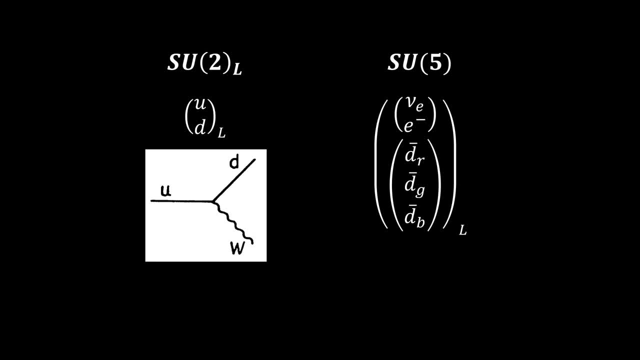 When up and down quarks are put in SU2 doublets, the gauge bosons W± act as raising or lowering operators, causing transitions between up and down. Similarly, when quarks and leptons are put into an SU5 multiplet and the SU5 theory makes a gauge theory, SU5 gauge bosons arise. Some of them are: 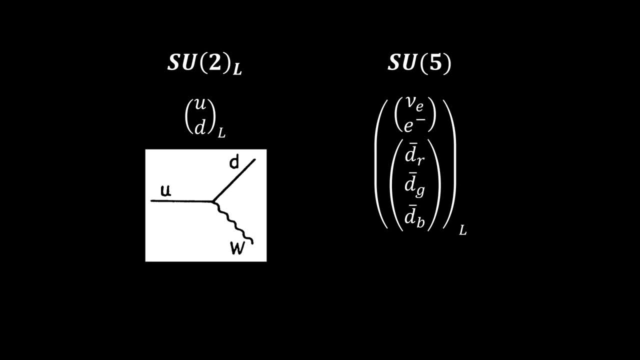 the familiar ones γ, W±, Z and gluon. but the rest can cause transitions between quarks and leptons among the states in the 5-plet containing the lepton doublet and the d-bar color triplet. If the quarks in a nucleon can turn into leptons, then the proton can decay. 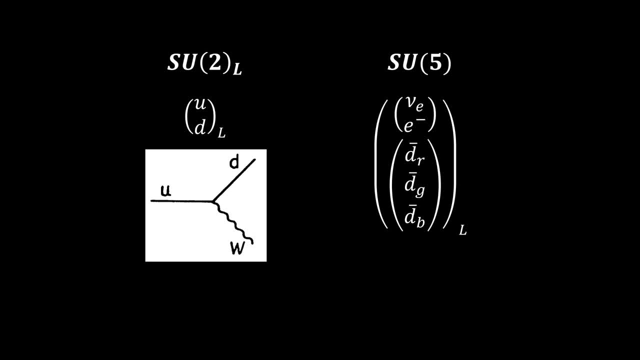 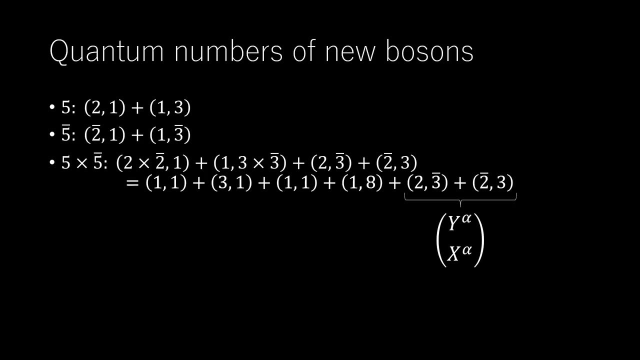 and baryon number is not conserved. We expect quarks to turn into leptons in a way that conserves color, since SU3 is a part of the SU5 invariant theory, and electric charge will be conserved just as it is in the standard model To find the quantum numbers of the new bosons. 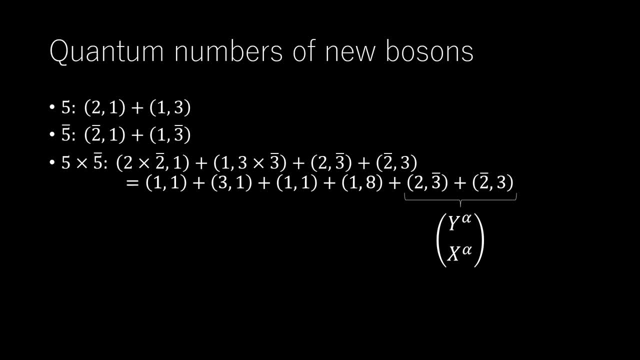 we can proceed. For SU2, for fermions in doublets to couple to gauge bosons, we have 2 cross 2 bar equals 1 plus 3 and the Ws are in the triplet. For SU3, it becomes 3 cross 3 bar equals 1 plus 8, and the 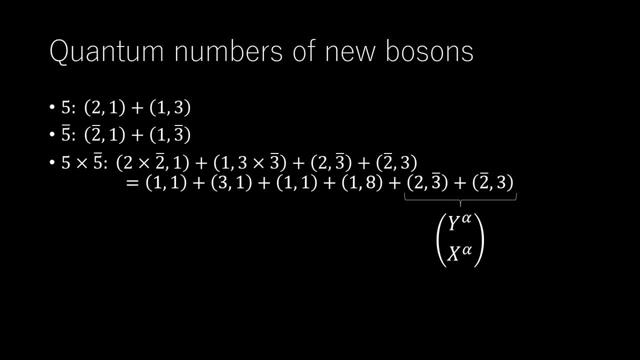 gluons are in the octet. For SU5, it is 5 cross 5 bar equals 1 plus 24.. We can trace the quantum numbers by remembering that 5 contains 2,, 1, and 2.. For SU5,, it is 5 cross 5 bar equals 1 plus 24.. 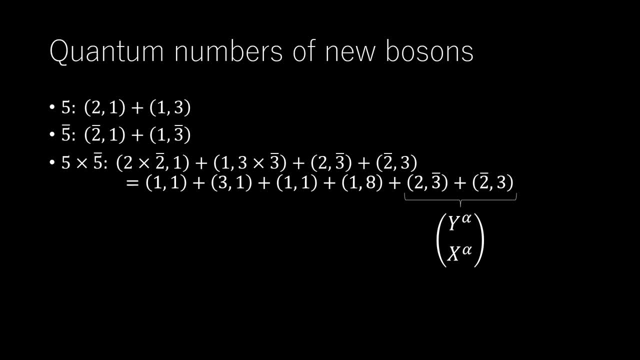 Then for 3- Ohh, anotherしょanger than 3, it becomes 1,, 1 or 3.. Where the quantities in brackets are SU2 multiplicity, SU3 multiplicity. For 5: Mohndt 책. 5 bar contains 2 bar equals 1 plus 1, 3 bar equals two bars. 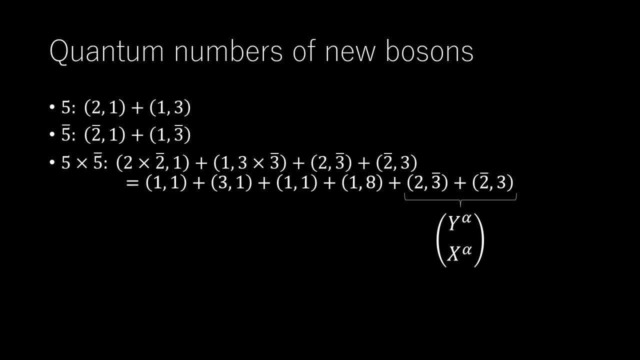 So 5 cross 5 bar equals 2,, So 3 vale work. so 5 cross 5 bar includes 2 cross 2 bars equals 1 plus 3. Hey, it gegeben like. maintenant. It valelooks like this: plus 3, 1, plus 1, 1, plus 1, 8, plus 2, 3 bar, plus 2 bar 3.. 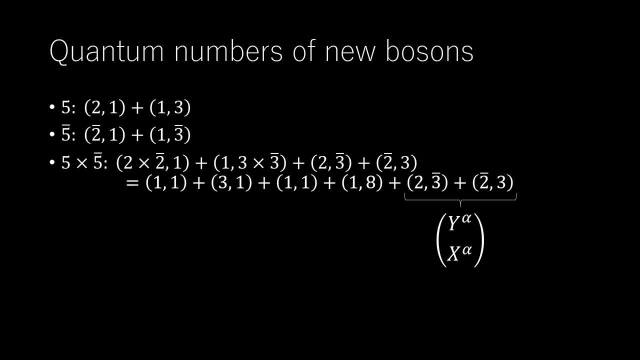 The singlet under both is the 1 in 1 plus 24, and changes no quantum numbers. The 3, 1 and 1, 1, are the W mu, I and B mu, and the 1, 8 are the gluons. 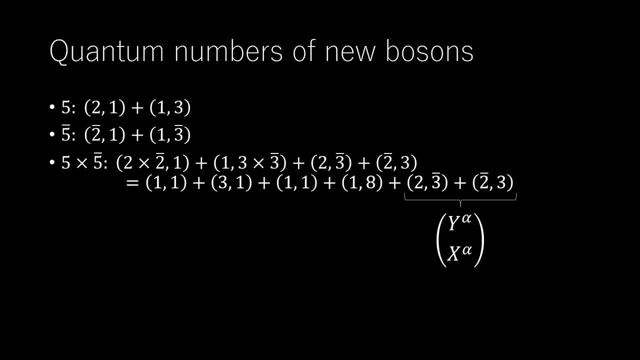 The remaining states an SU doublet of color triplets and their antiparticles are the new bosons. They are usually denoted as Y- X with electric charges, Q- Y equals minus 1 third. Q- X equals minus 4 thirds. 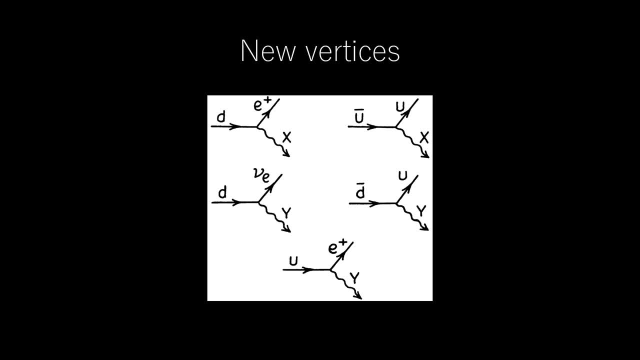 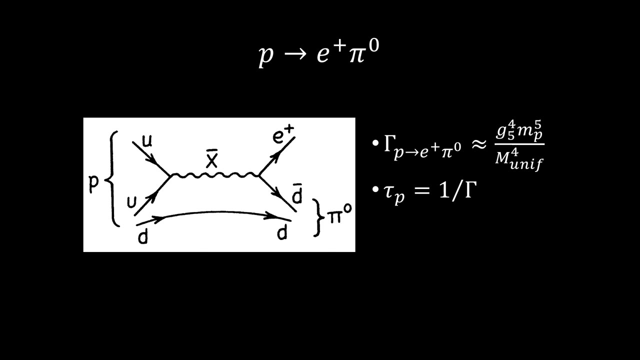 The new vertices in the theory are shown in figure. As always, the lines can be reversed by replacing particle and antiparticle. Any process can occur that can be drawn with the vertices of the standard model plus these. In particular, one possible transition is shown in figure. 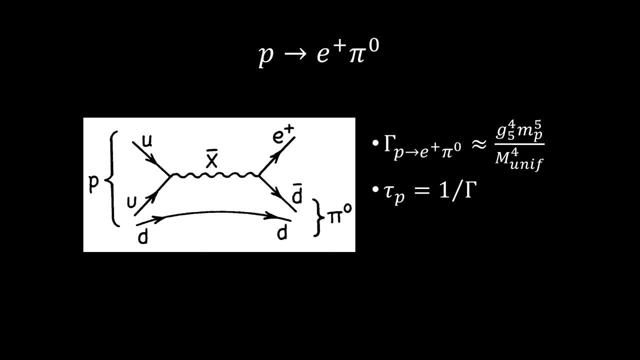 If X gives rise to the decay, proton goes to positron plus pi 0, which is not allowed in the standard model because the diagrams cannot be constructed, but is allowed here. Our usual technique to estimate the width is not expected to apply here because hadronic 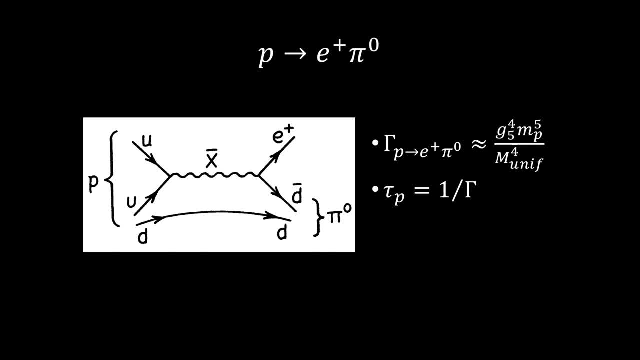 binding effects are involved. Since we expect M X to be large and presumably of the order of the grand unification scale, we only need a very crude answer: The matrix element must have a factor G 5 squared over M X. We only need a very crude answer. 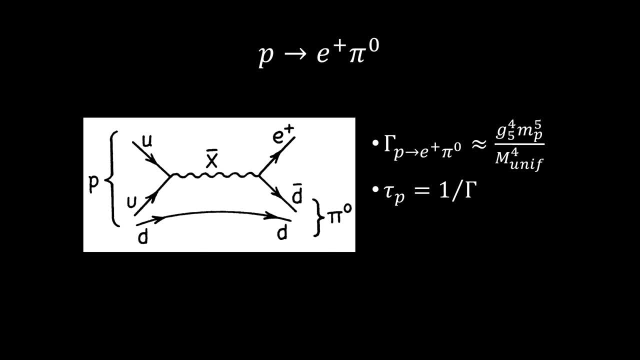 The matrix element must have a factor G 5 squared over M X. So the width has a factor g5 to the 4th over munif to the 4th. By dimensions, the width must be proportional to a mass, and the only mass that could be 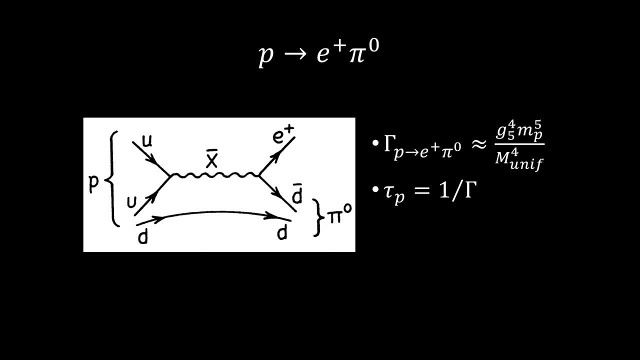 relevant is the proton mass, mp, Thus up to a numerical factor. the width γ must be about g5 to the 4th, mp to the 5th, over munif to the 4th. The numerical factor will be proportional to the probability of two quarks being in. 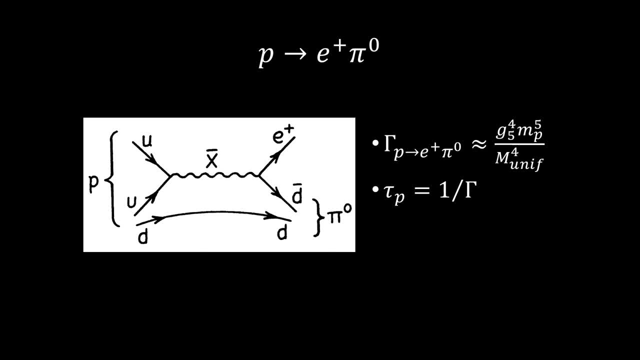 the same place so they can annihilate, which is significantly less than unity. So the lifetime τ equals 1 over γ- will be even longer than indicated by the widths shown Numerically. since τp varies as munif to the 4th, it is very sensitive to the value. 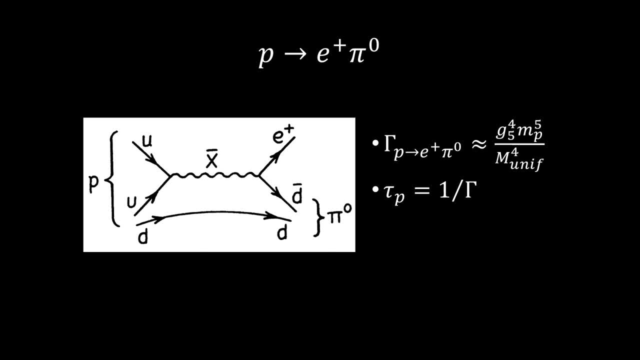 of munif, For munif equals 5 times 10 to the 15th GeV, we get τp about 10 to the 31st years. The universe has a lifetime of about 10 to the 10th years.